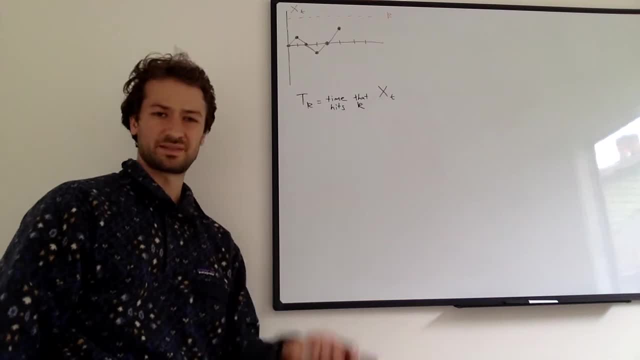 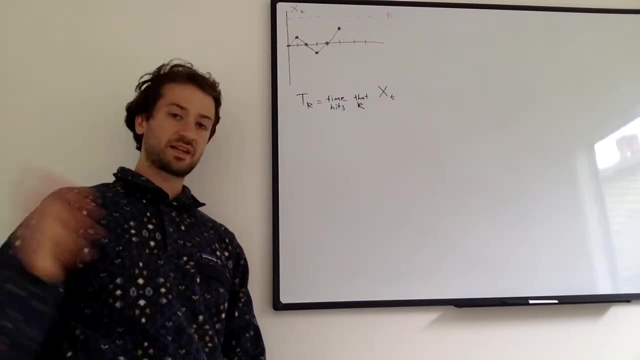 Like you know, we can think of like running a simple random walk a bunch of times and each time we have kind of a different value of time that it takes to maybe hit some three hits, seven hits, 15 hits, whatever. 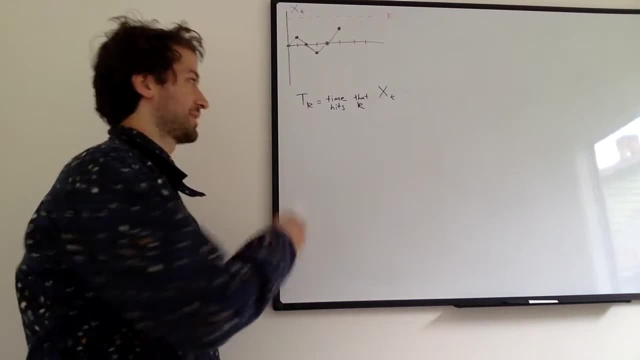 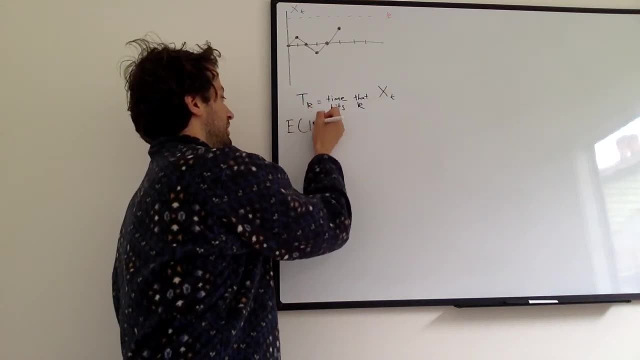 T is greater than zero, especially if actually T is greater than K, I guess. but we'll get to that in a second, And we are concerned with the expected value of T sub K, So the expected amount of time it takes us. 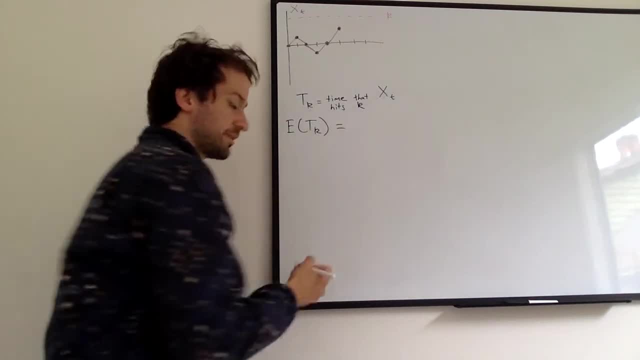 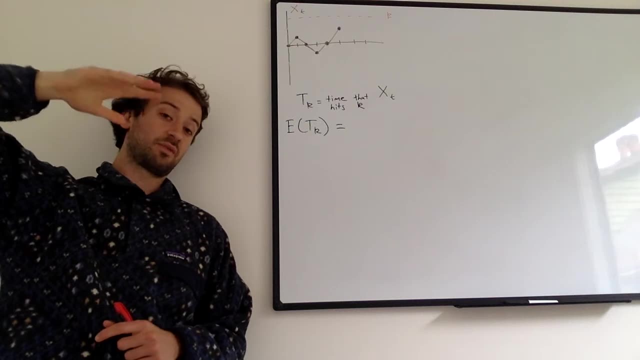 to hit K. basically, And similar to the previous video, we can kind of think of getting up to level K as getting to level one a bunch of times, right, So to get to step five, we basically have to get to step one. 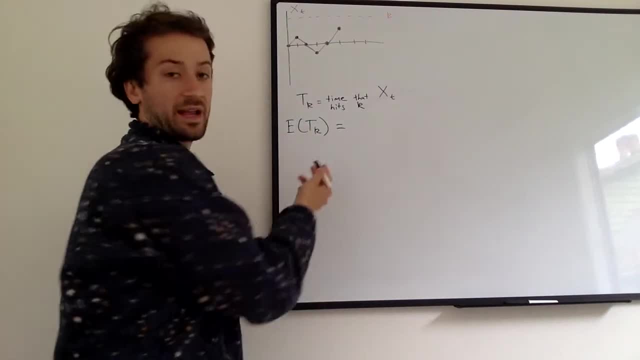 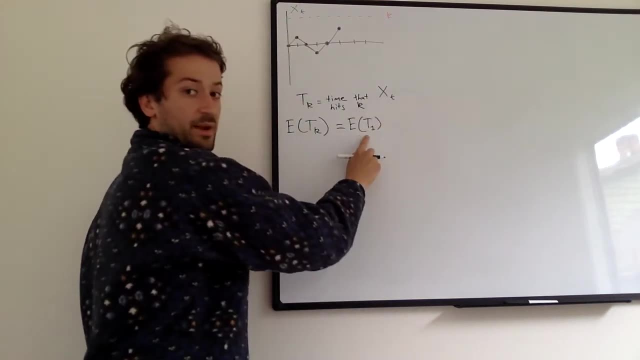 and we have to do that five times. So when we can break out expected value of T sub K, we can just say: that's the same as the expected value of T one, which is the expected amount of time it takes to get to step one plus E of T one plus dot dot dot. 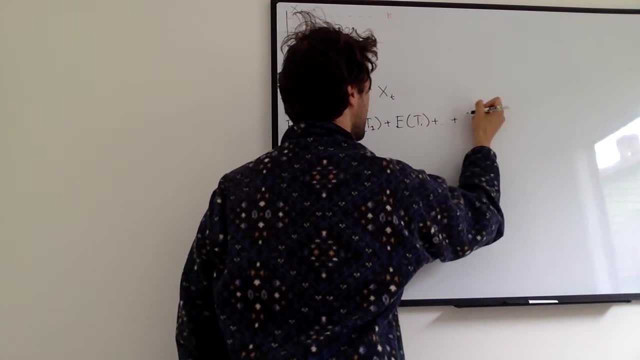 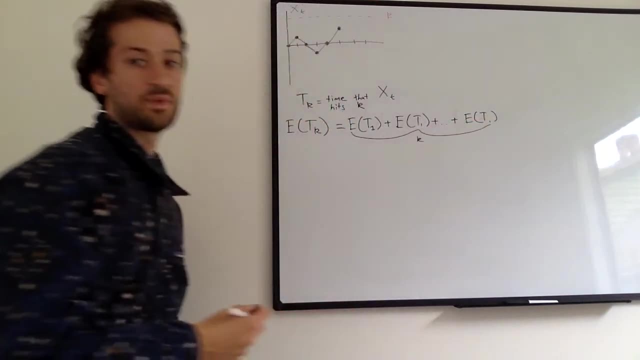 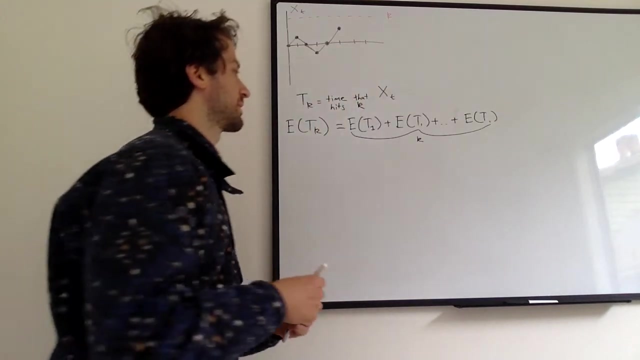 plus, sorry, plus E of T one, and I'm gonna have K of these terms, right, Because I get to one, then I get another one, and I get all the way up to K and the intervals are independent. so it's kind of okay to think about this. 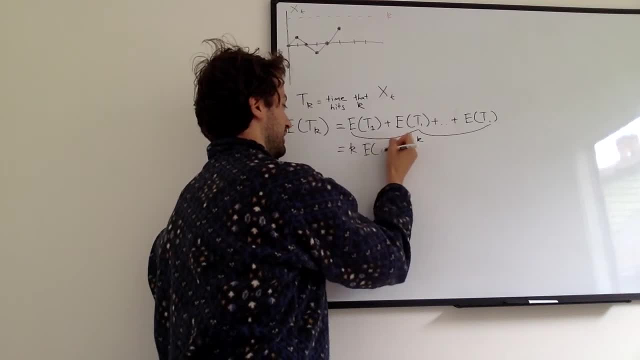 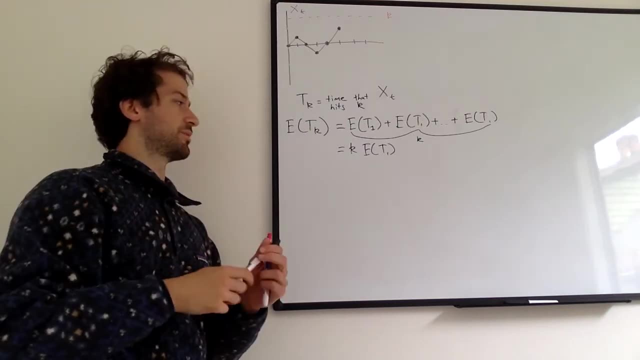 and if I just want to simplify this, it's K E T right. And what's really nice is that E just like in the last video, with probabilities, expected value of T one is way easier to find than expected value of T K. 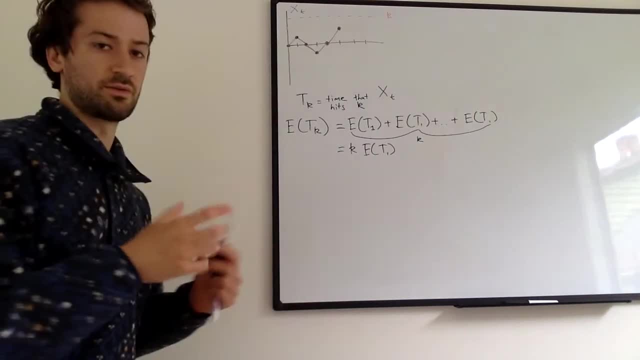 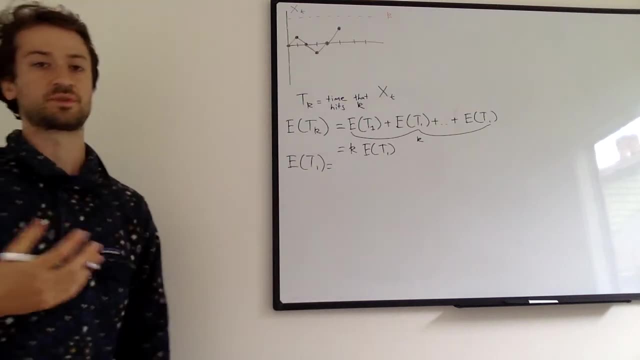 Okay, so we're actually gonna, if you're just coming from the last video, we're gonna do a very similar approach, right, A very similar approach. so expected value of T one. We're gonna condition on the first step. so first step analysis and say what. 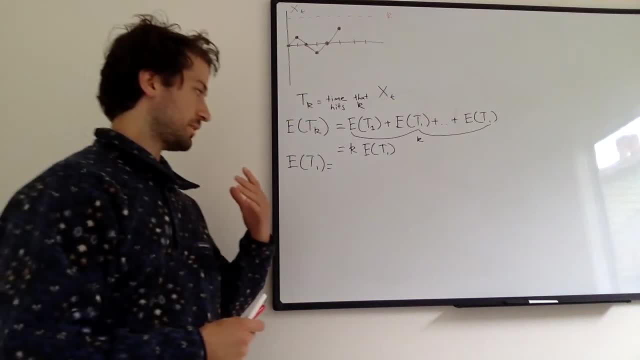 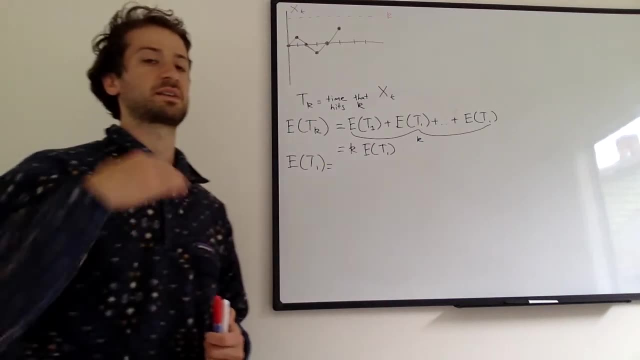 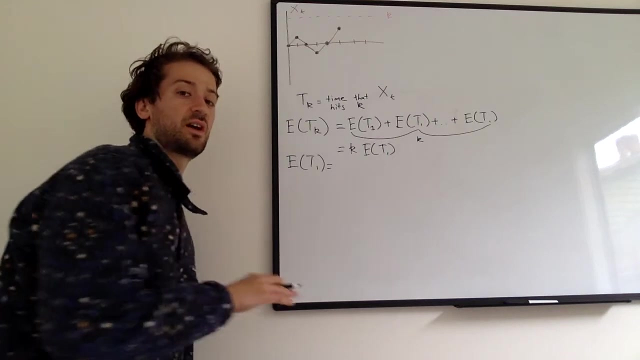 based on what happened in the first step. we can kind of break the world into two pieces, probability weighted by what those worlds are, and then think of the expected value of hitting one, based on those two outcomes. So it's slightly different, so we're gonna condition on the first step. 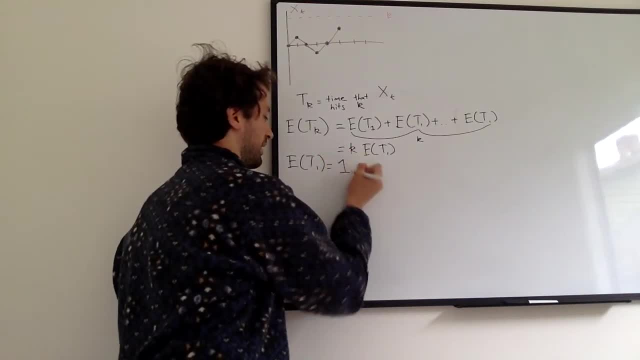 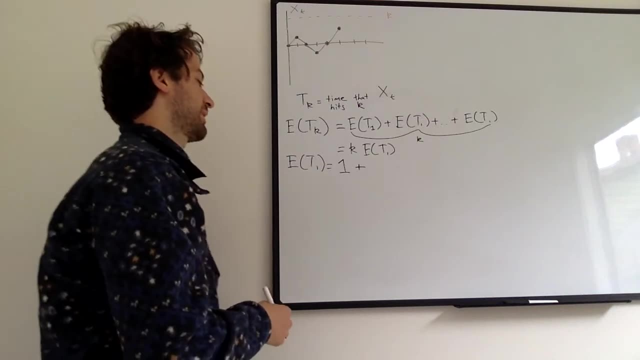 which means we've already taken one step, which means automatically we have to put a one in here so that we have one plus, because we've already taken the first step and we're conditioned on that and we kind of know that's already occurred. 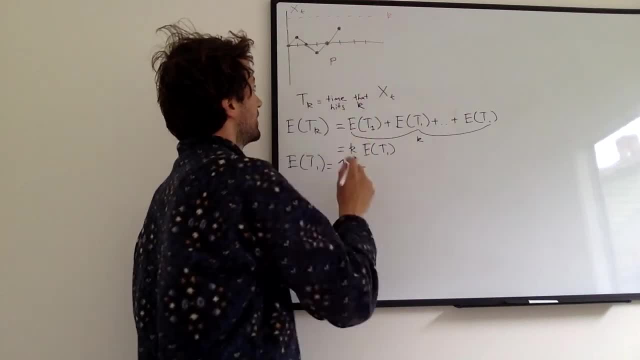 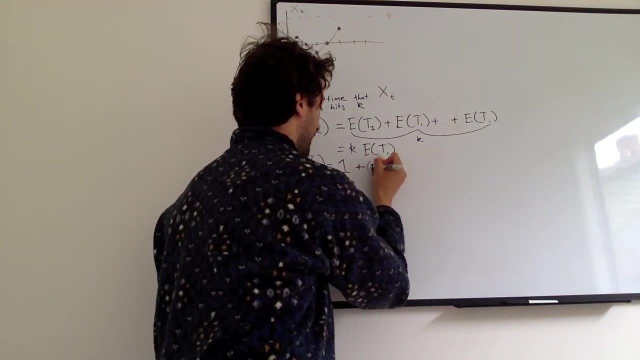 So we have probability P. I should put it up here probability P. we have probability P of going up right on the first step from zero right. So probability P, and if we go, if we go up on the first step from zero right, 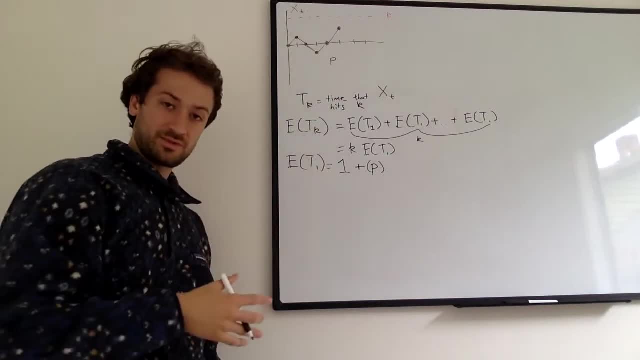 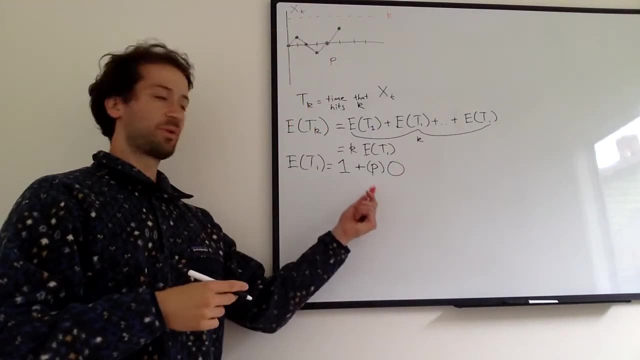 our new expected value of the time it takes to go to step one is just gonna be zero because we've already reached step one. So probability P that our expected wait time is now zero, so that this term just can't step. 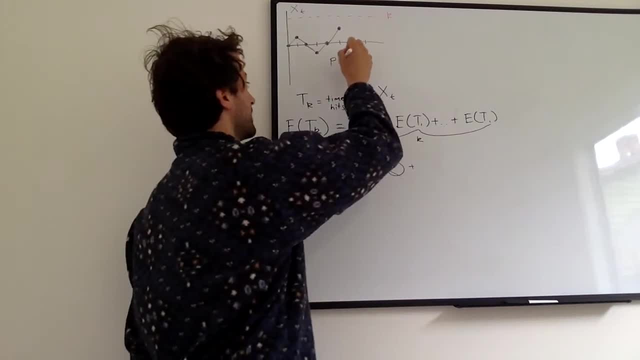 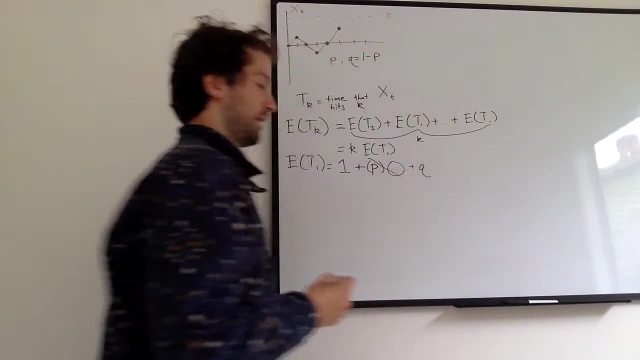 And then we have probability Q. Q is one minus P. we'll just write that, for we just kind of use that for shorthand. so we have probability Q of going down, so down the step to negative one, and then we have to go up two steps to get back to one. 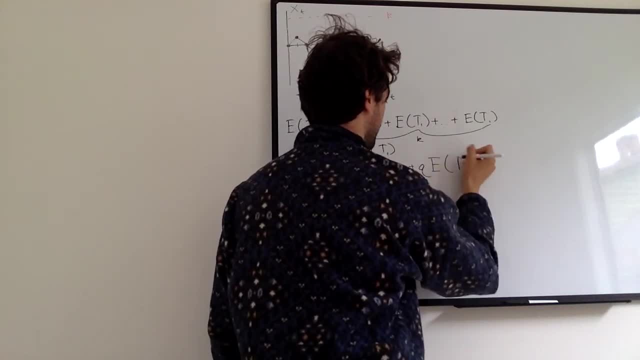 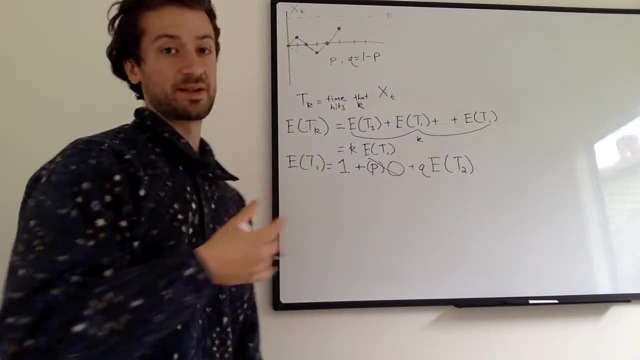 right And this now: we now have the expected value of T two right, where we basically went down a step and now we have to go up to zero and then to one. so we need the expected value of the time it hits to hit. 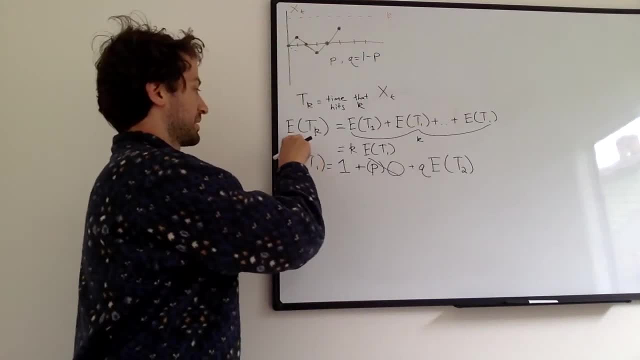 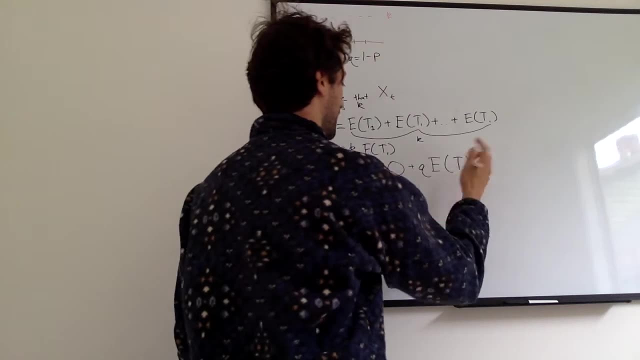 the time it takes to hit two, And we can use this formula: the expected value of T sub K equals K expected value of T sub one. plugging in two for K, this just becomes one and we get a two here. 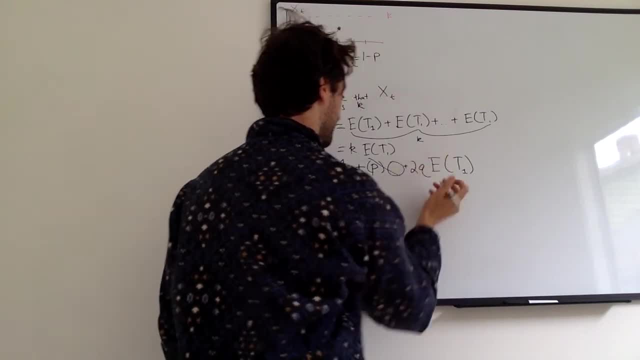 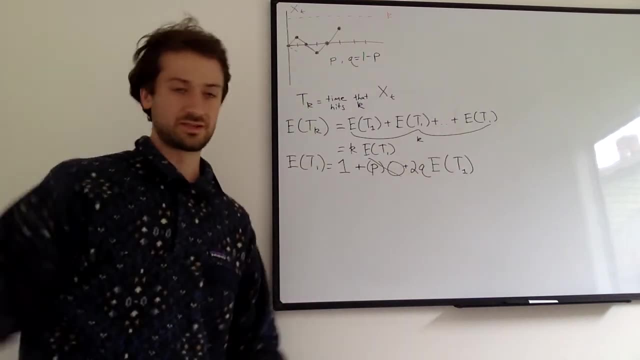 so we're gonna put the two up plus two. So I basically just took the two and put it out here. it takes two single steps to get to the two steps overall, So we get this nice. I'll just write it out without that. 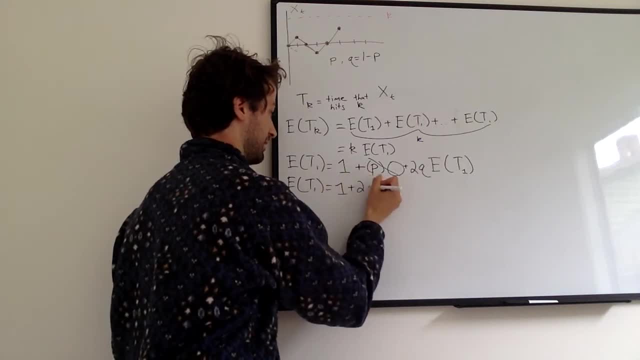 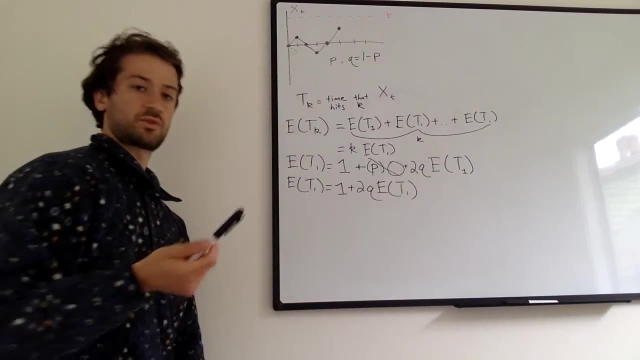 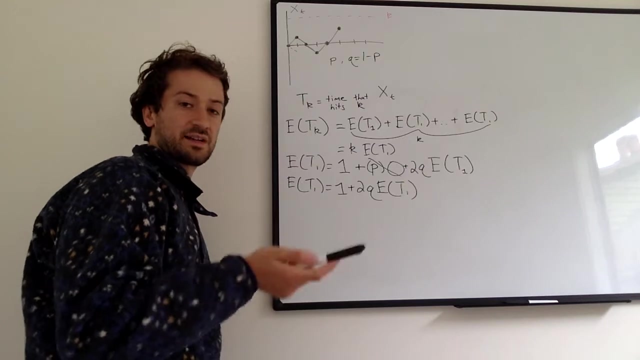 zero term equals one plus T sub one, And now we have two quantities that we we're solving for expected value of T sub one. Everything in this equation other than expected value of T sub one is a constant. So now we can solve for expected value of T sub one. 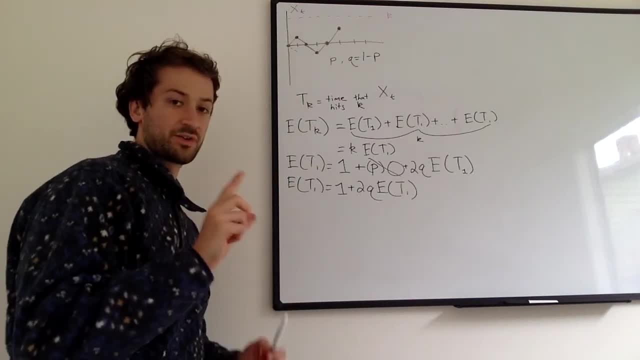 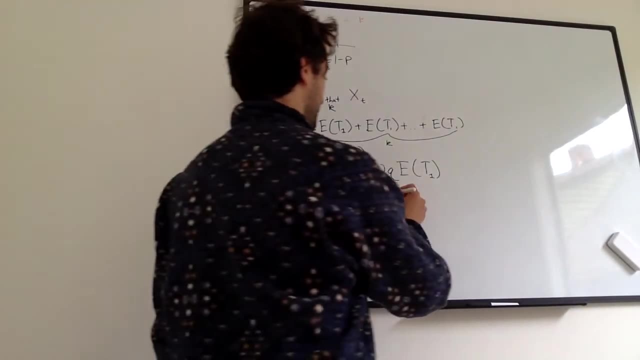 which is really neat. So first we're gonna do kind of a funky case. We're gonna do the case I'll do it over here. actually Let me turn this a little bit. We're gonna do the case where P equals Q equals one half. 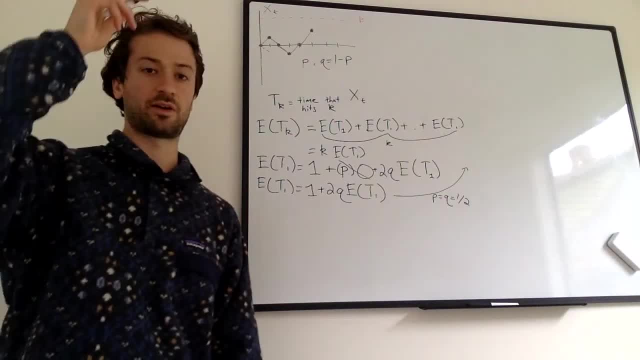 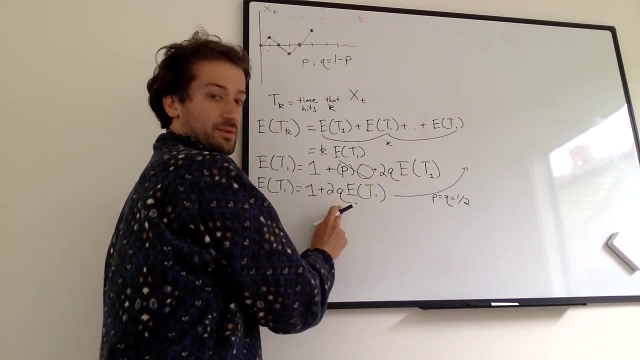 So P is one half, Q is one half. it's a symmetric random walk. it could go up or down, equal probability. So if we plug in one half, Q equals one half of this, this just becomes one two times one half is one. 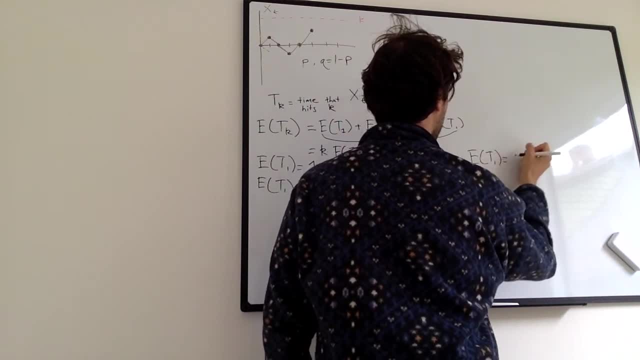 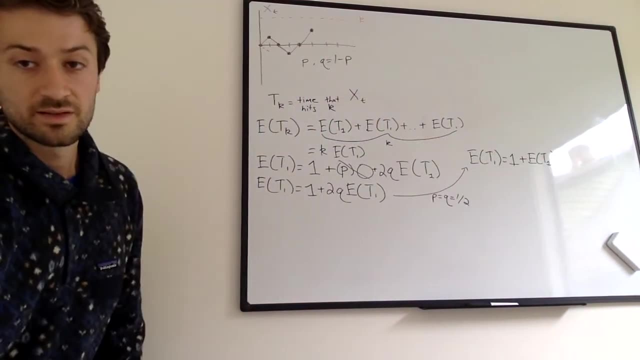 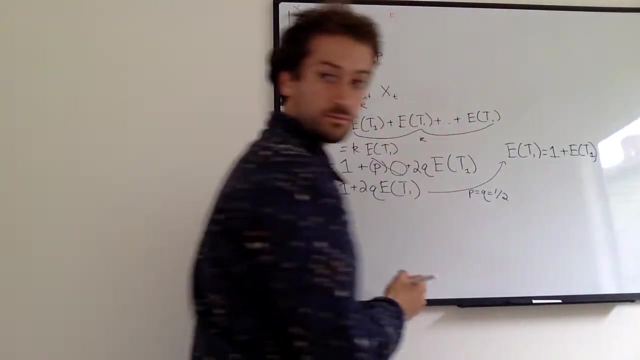 So we get expected value of T sub one equals one plus expected value of T sub one. So this is a little bit in the glare, A little better. So that's kind of weird. We see expected value of T sub one is one plus expected value of T sub one. 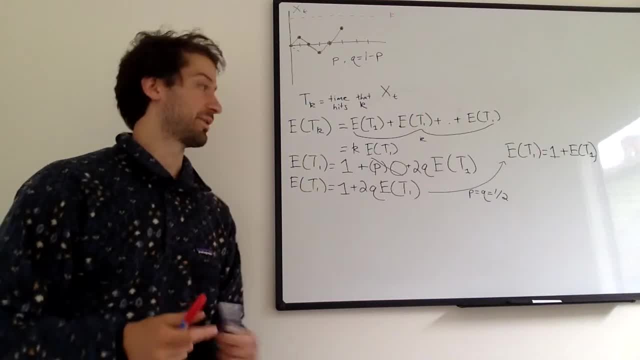 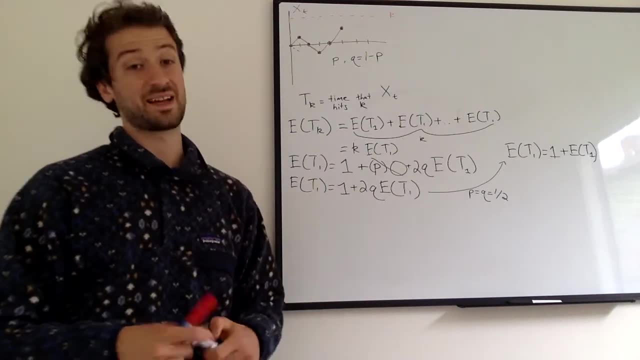 That's like writing X equals one plus X. That's kind of weird. If I subtracted expected value of T sub one from both sides, I get zero equals one. That's incorrect. So what? our answer here is actually- and this is really funky- 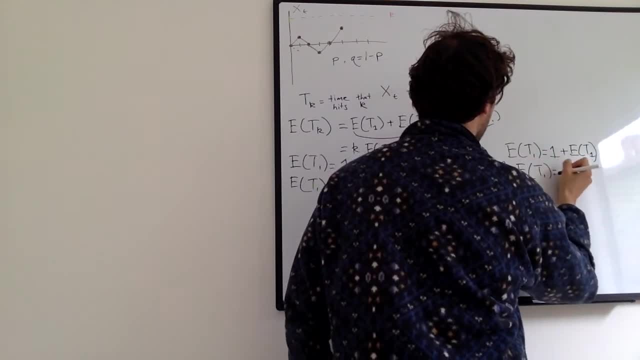 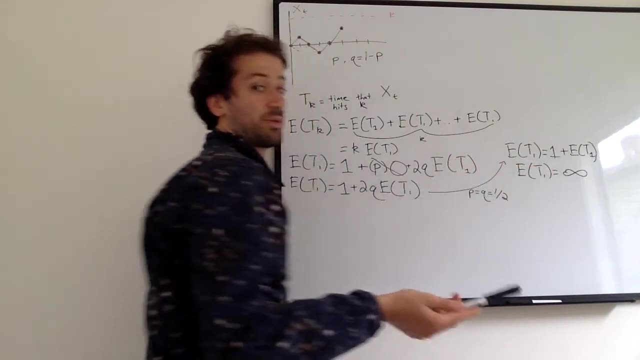 but what our answer is is: expected value of T sub one equals infinity, And you can kind of convince yourself that this works, because infinity is the same as one plus infinity. One plus infinity is still infinity, So then it seems kind of weird. 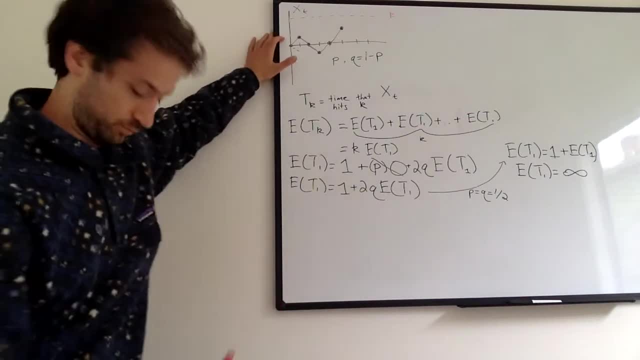 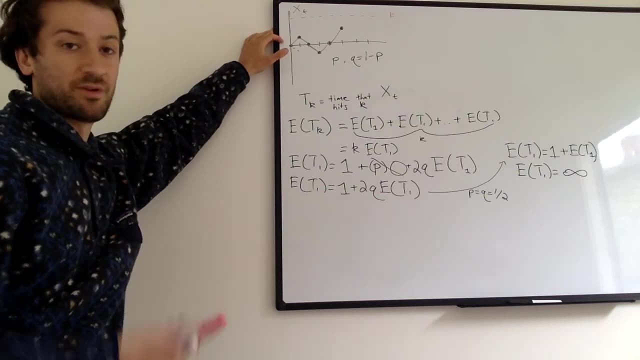 The expected value of getting to one like one is just one step away from zero. Like that's the. I have a little door stopper. I just kicked it. One is just one step away from zero, So why is it an expect? 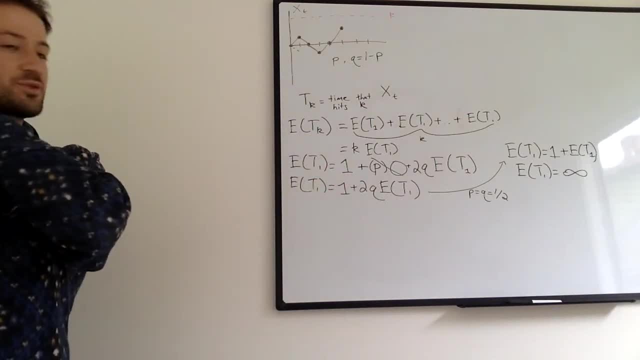 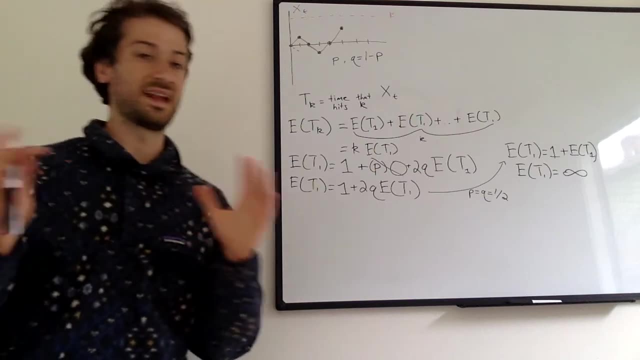 why does we expect, on average, it will take. you know why? on average will it take infinity time to get to one step above zero? It's just one step away. Well, to think about that is obviously, in half the cases it's just going to take one step to get to one right. 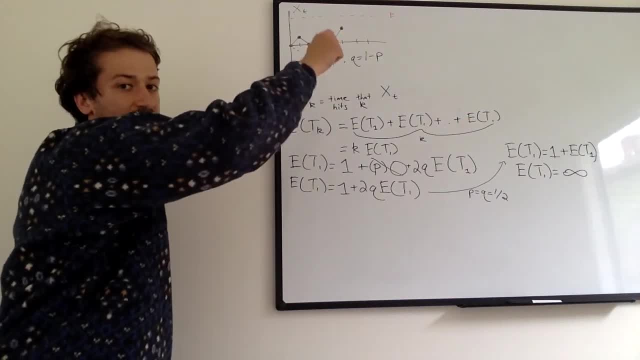 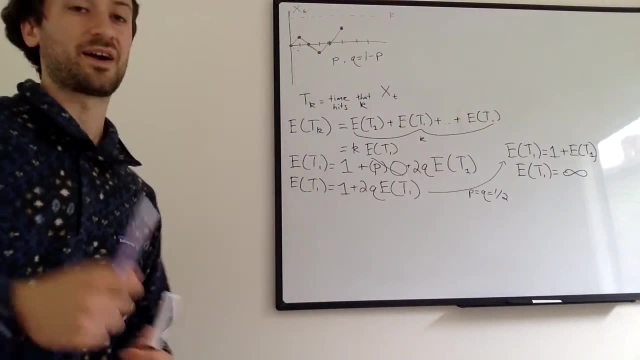 And most of the time, even if you drift down a little bit here, eventually the symmetric random walk will bounce up and hit one. However, there are cases where it will take an infinite amount of time, you know, and thinking about infinity is not really the purpose. 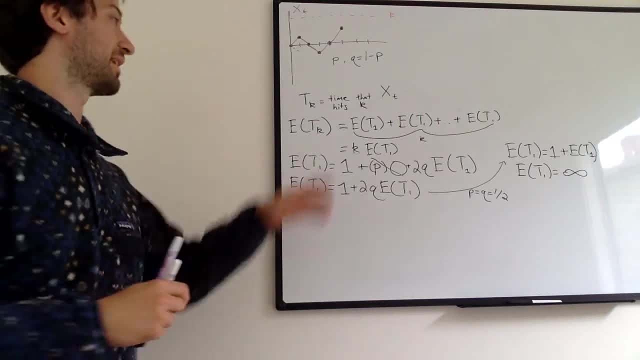 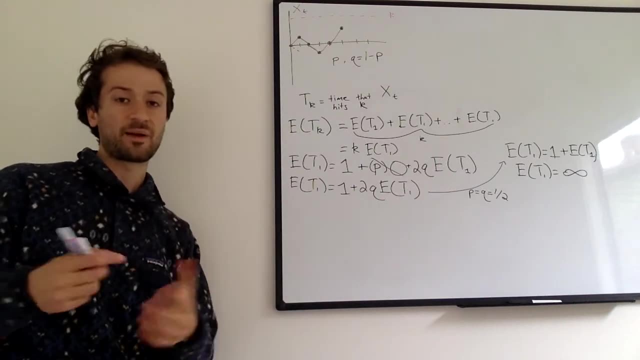 of this type of stuff, But there are some cases where we'll take an infinite amount of time, where the random walk gets far enough away from one down. you know down here. however, it'll take an infinite amount of time, And because there's some cases, 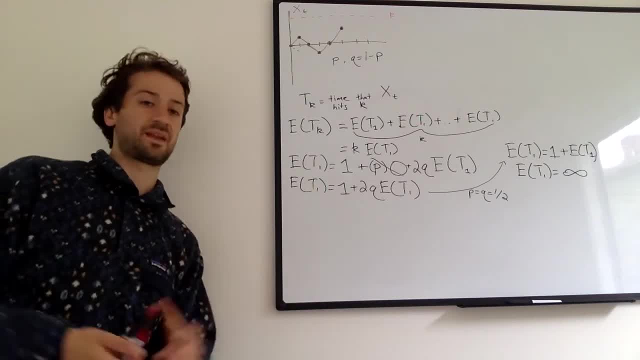 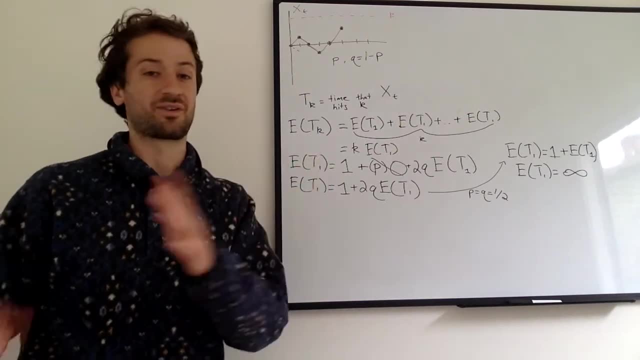 where we'll take an infinite amount of time. the expected value is infinite And that's kind of weird because you have- most of the cases are a very finite, you know small, amount of time. Half of the cases are one step away from zero. 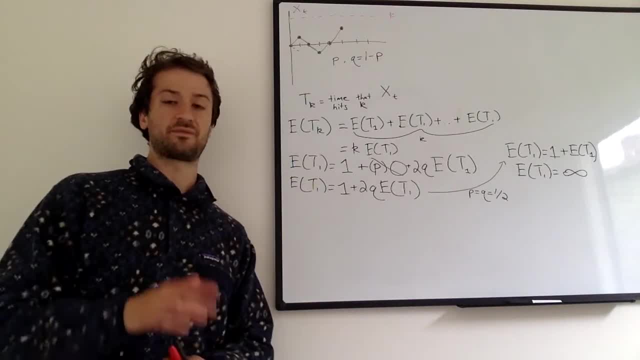 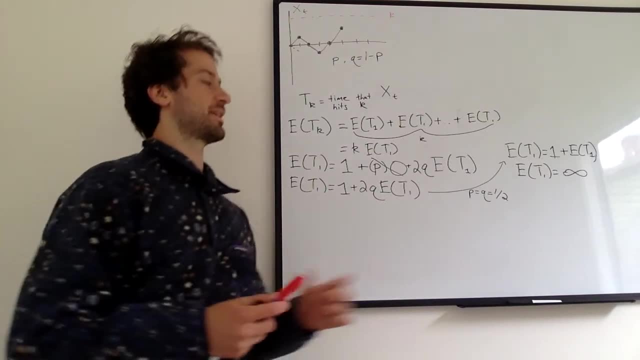 Half of the cases are one, But if you throw one infinity in there, everything kind of becomes infinity. So that's kind of a- you know not super mathematically sound, more kind of an intuitive explanation for that. But that's why we see this really weird result. 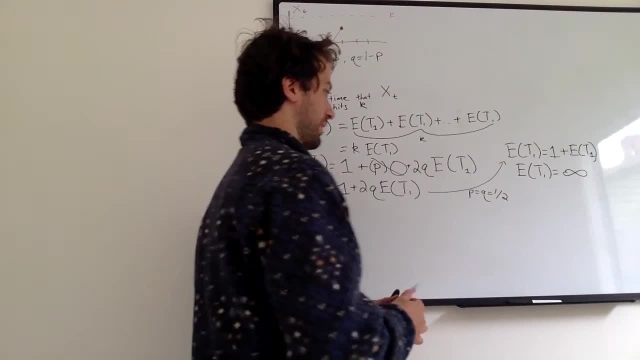 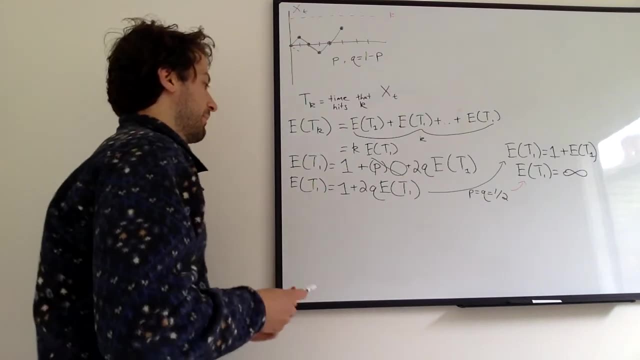 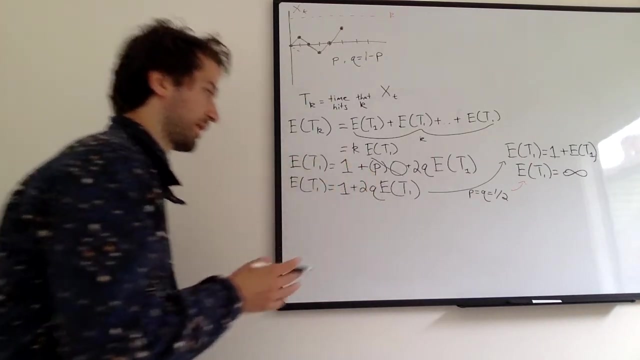 When P and Q are one half, when this is a symmetric, random walk, you get expected value of T equals infinity. So really weird. Let's return to the case- most cases- where P and Q are not equal to one half. So now we don't get this weird: X equals one plus X. 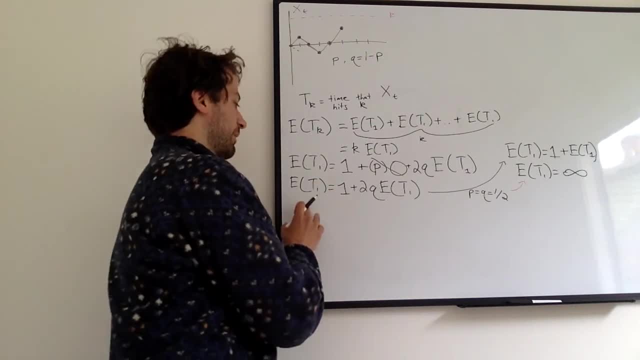 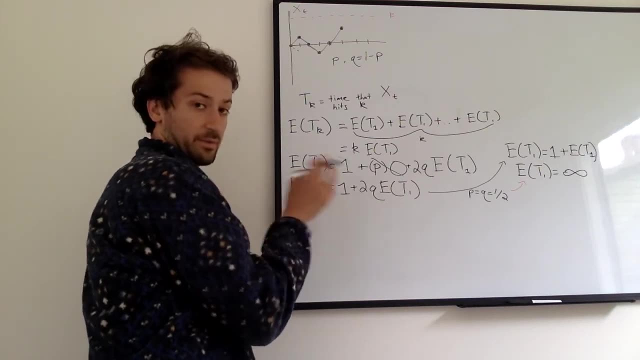 Let's just go ahead and solve for the expected value of T sub one. So I'm gonna subtract from both sides, I'm gonna subtract the two Q and I'm gonna get. so I'm gonna factor out, So I'm gonna get expected. 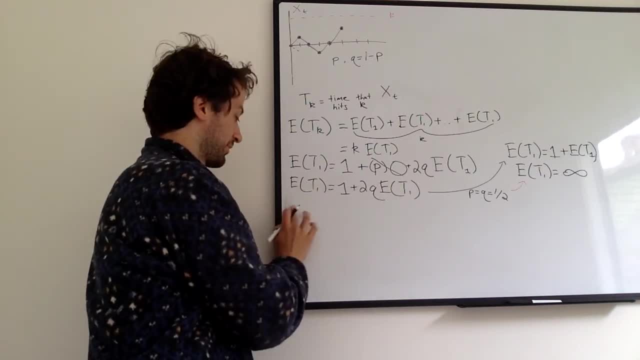 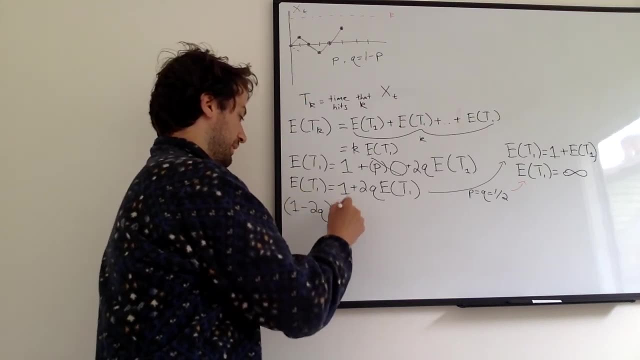 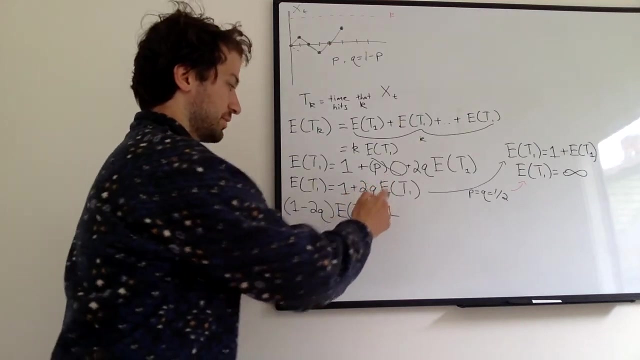 Look, I'll basically do subtracting the two Q E T plus one, And then I'm gonna factor out the E T plus one, E T sub one, getting one minus two. Q E T sub one equals one. Okay, So I just moved over the two Q E T sub one. 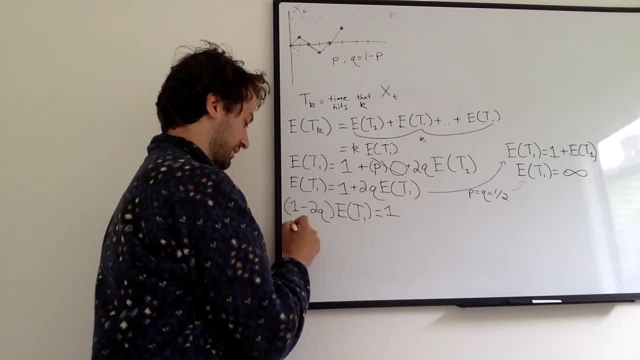 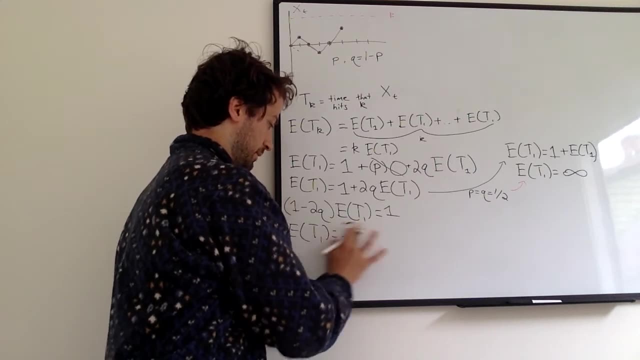 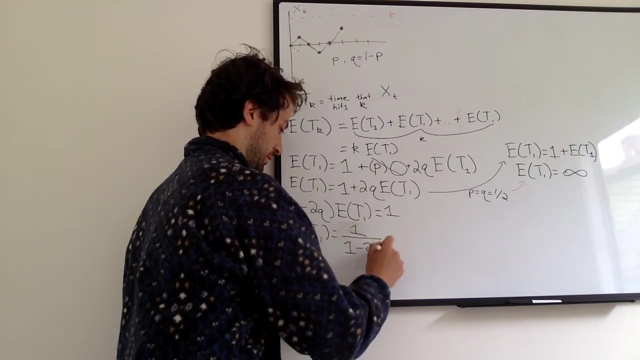 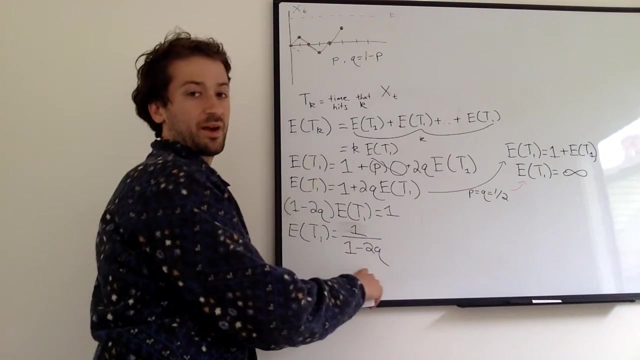 factored out E, T sub one, and I get this, And then it's just an easy division And we don't have time in this video to simplify this. but I promise you, if you expand one minus two Q, if you plug in one minus P, 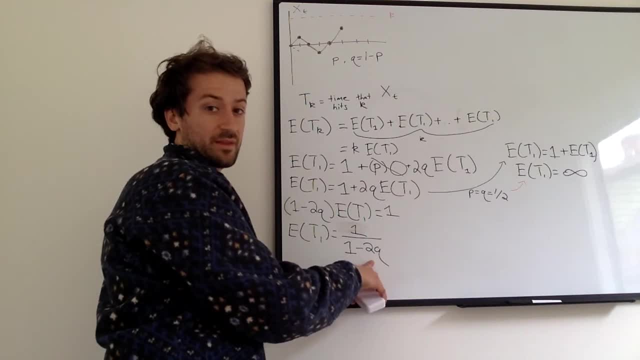 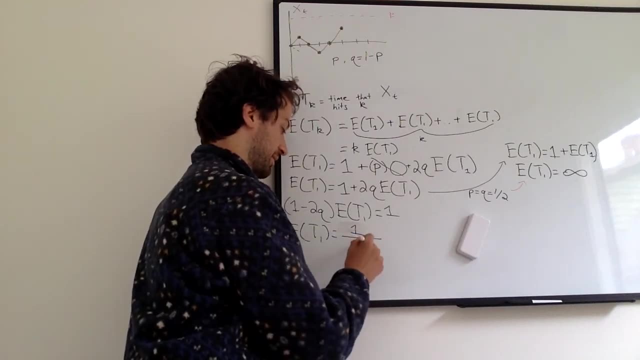 this is like good arithmetic exercise. You plug in one minus P to this. So one minus two times one minus P, you're gonna get P minus Q. It's gonna simplify one minus Q, P minus Q. So again, we're not gonna show it here. 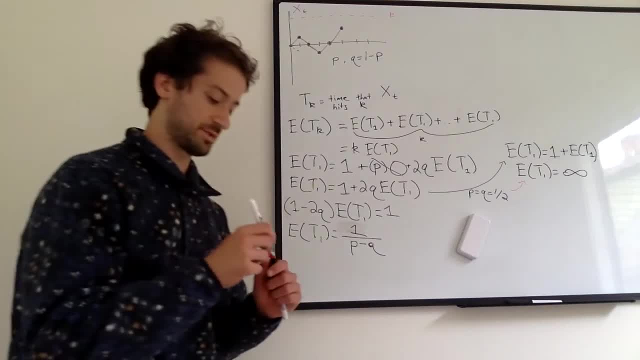 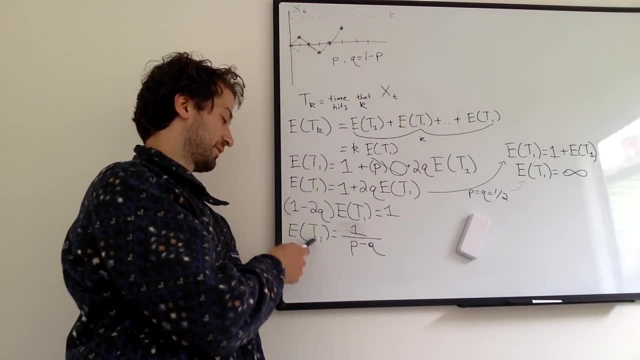 just because we don't have that much time, Check it for yourself. I promise it works out. Yeah, one over P minus Q, So that's pretty cool. We get, like we've solved, expected value of T sub one. That's the amount of time we expect it to. 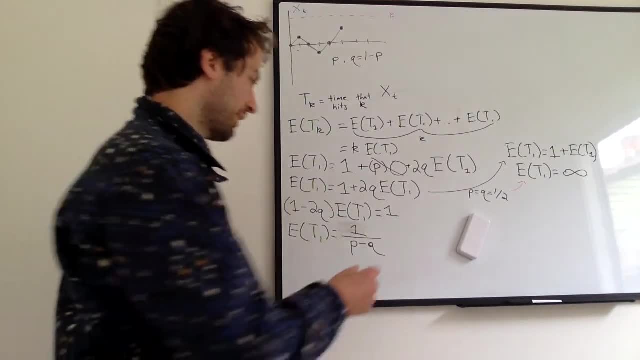 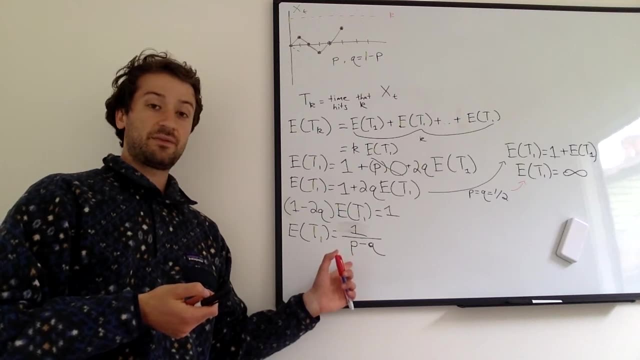 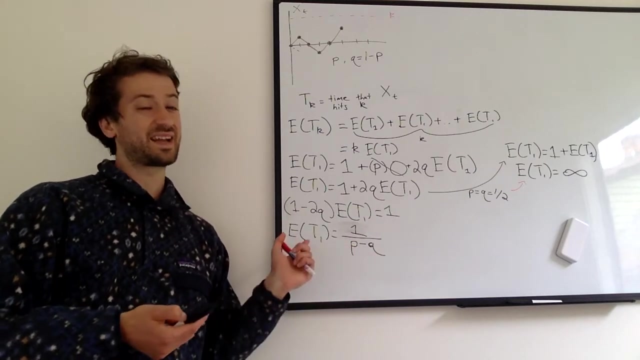 to get. So we hit one. However, maybe the kind of sharp eyed among you have noticed, if P is less than Q, this is gonna be negative, right Cause we're gonna have P minus a greater value. negative: We get a negative expected value. 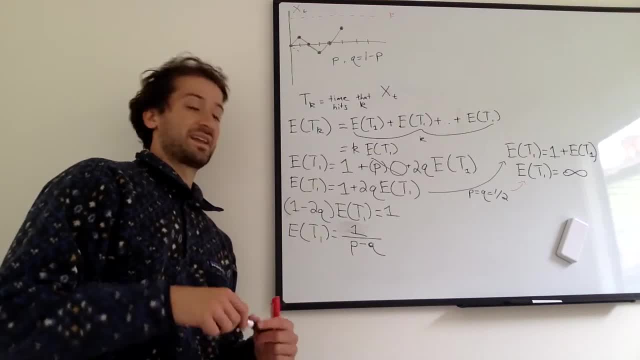 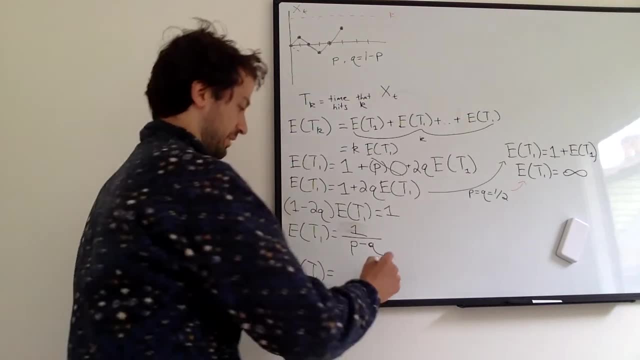 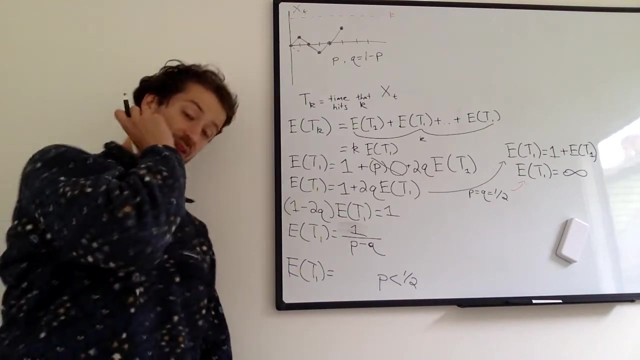 That doesn't really make sense, That doesn't seem to work, And that's so. in the case where, in the case where P is less than one half, So P less than one half, whatever you know, it's gonna be less than Q. 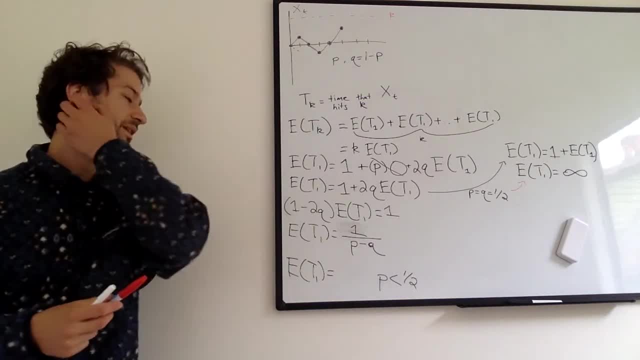 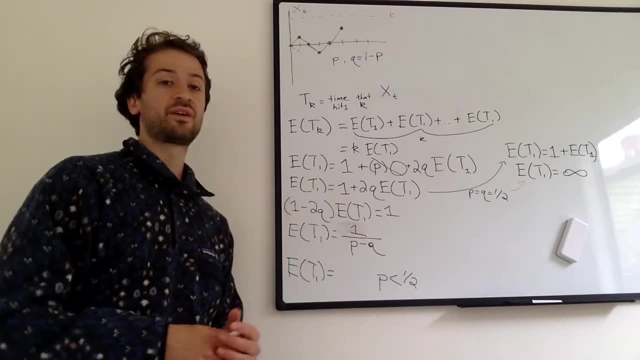 In that case, the expected value comes out as negative. That doesn't make sense, but that's a similar result to the result we got over here. Remember, in the previous video we saw that P is less than one half. There's a if P is less than one half. 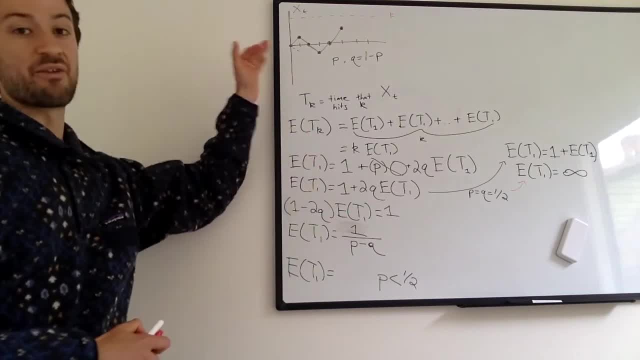 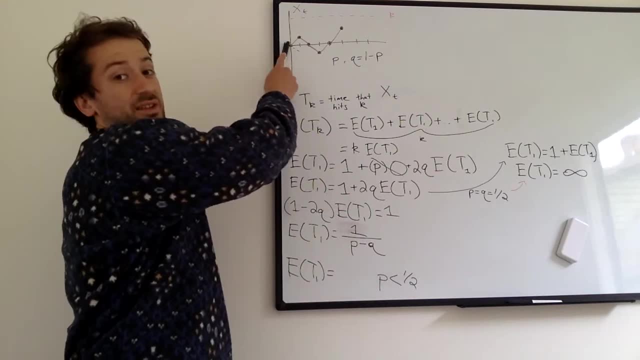 there is a non-zero probability. There's a probability that we never hit the value right. I think the probability is P over Q, you know. So if P is less than one half, there's a chance that we never, ever, hit one. 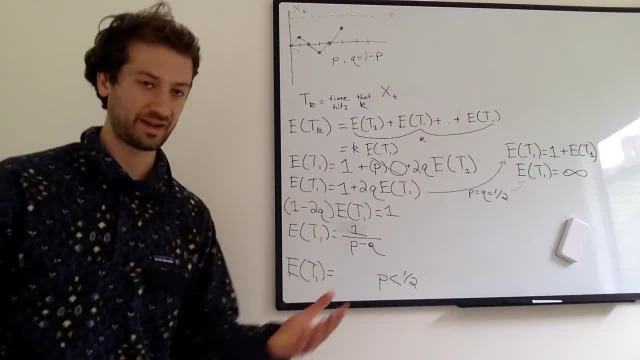 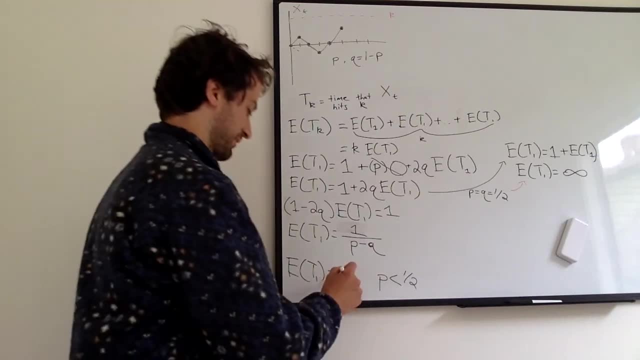 which means we will be waiting an infinite amount of time to hit one cause. we're never gonna hit it. Ergo, because at least some of the you know, at least some of the possible outcomes are infinite, this expected value is gonna be infinite. 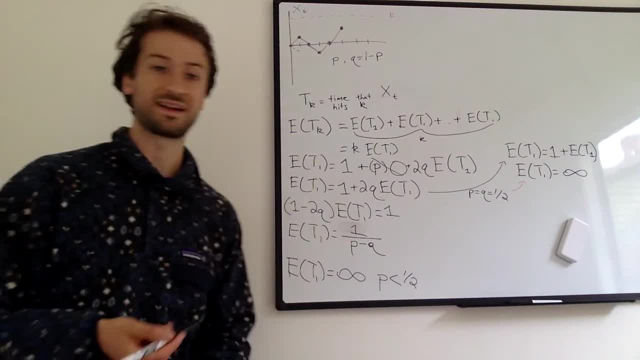 And that makes a little bit more sense. Like there's a chance we never hit it. There's a chance we're waiting an infinite amount of time. So the average is the expected value is gonna be negative, It's gonna be infinite. 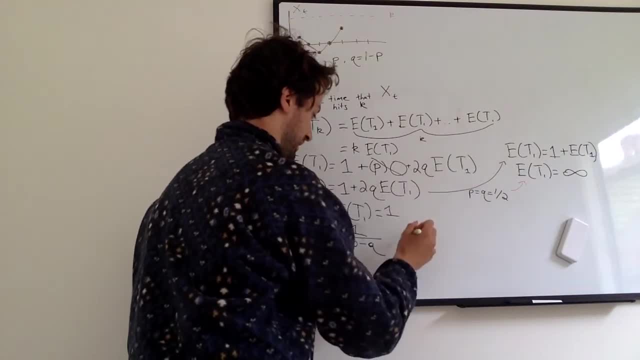 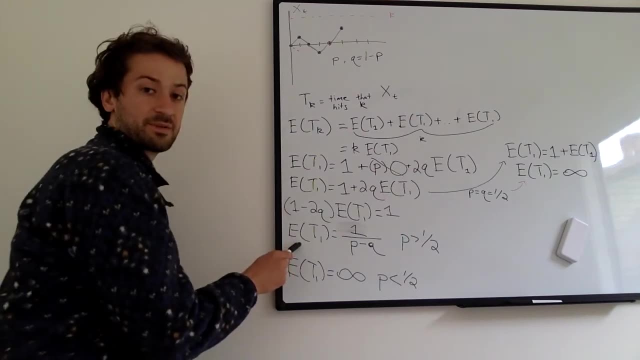 However, when P is greater than one half- not equal to, because we saw that equal to case- when P is greater than one half, we get this nice result And again, like we found, expected value of T sub one we can easily just plug in. we can easily make this a K. 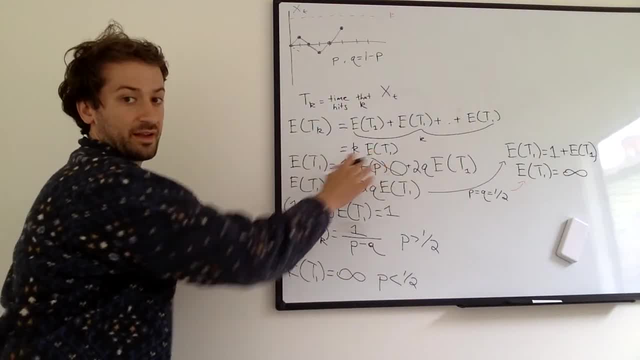 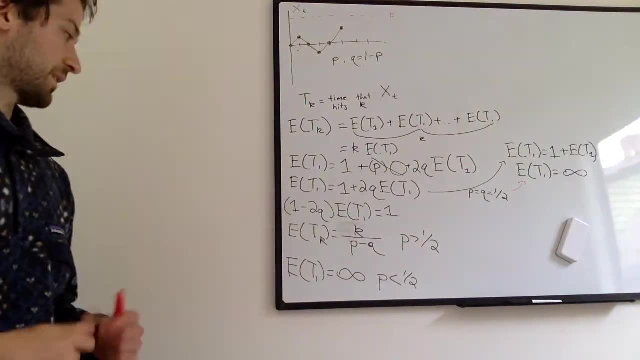 by using this formula: above expected value T sub K, It's K times expected value T sub one, which will multiply the right-hand side by K. We get K over P minus Q. So yeah, It's a similar derivation. We can look at some intuition on this term. 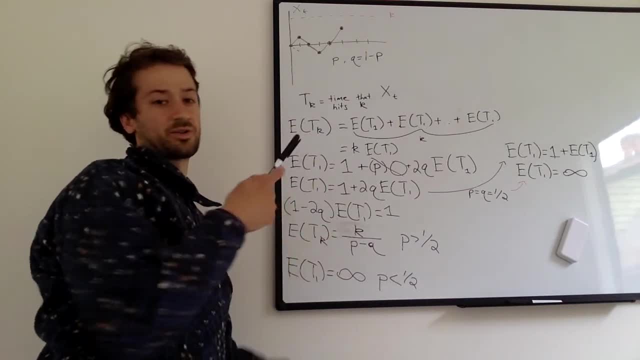 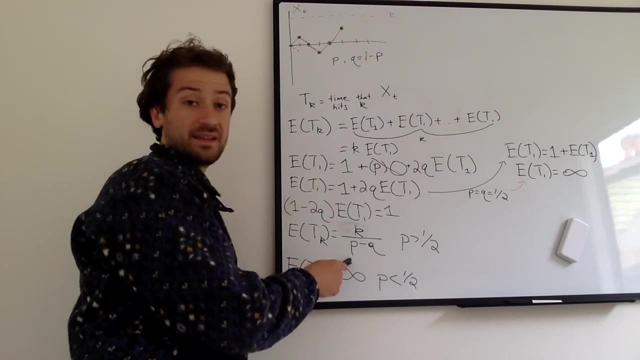 The larger that K is, the larger the expected value is, The larger the more time. if K is higher, we expect it to take longer to hit, which totally makes sense. The bigger that P is right. If P is larger, this denominator is smaller. 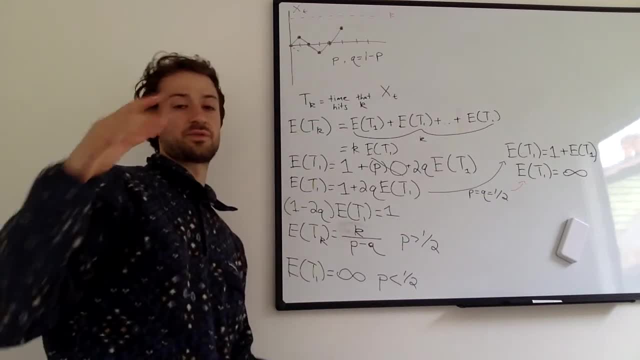 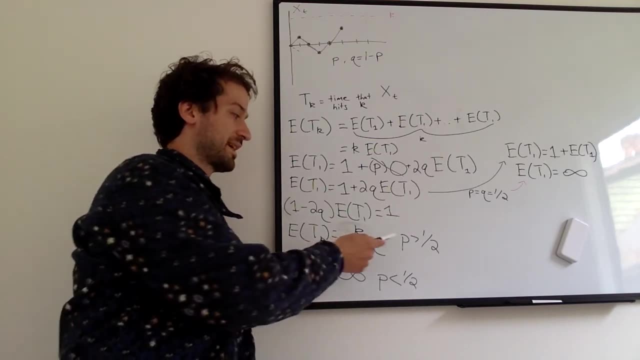 which means we're waiting less time. We're expecting to wait less time to hit K, which also totally makes sense, Because if P is larger, we should get there quicker And note that. you know, in this case- remember we saw when P is greater than one half-